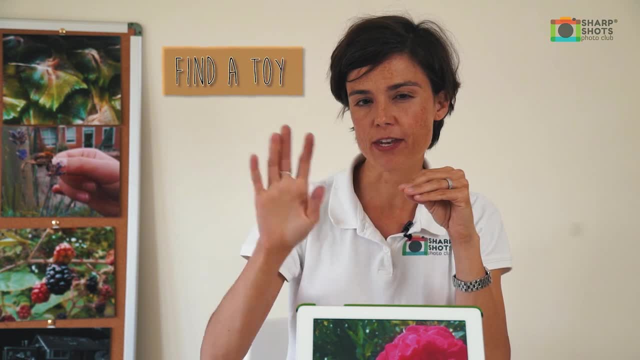 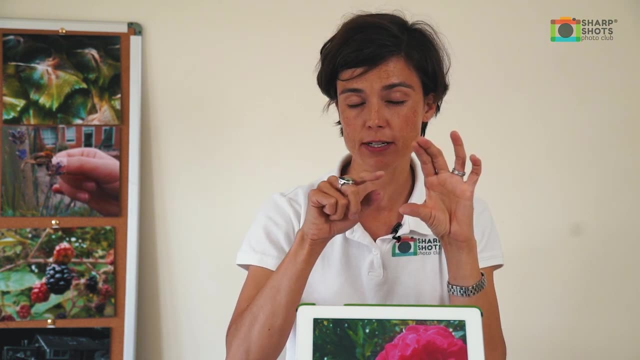 and I want you to put it on the left side of the frame. so then you have all the negative space in the rest of the picture showing off the room. but your toy is nice and sharply in focus, making sure that green square is on it, and take the picture. 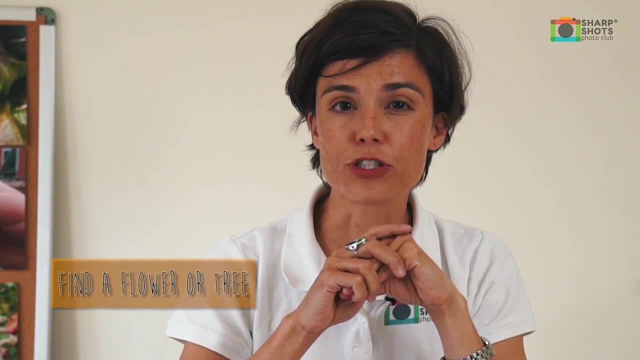 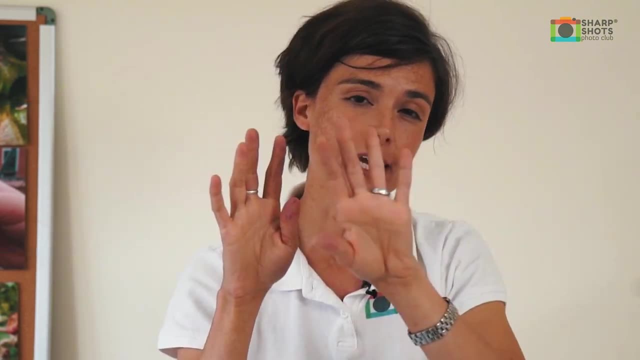 After that, I want you to do is to run off into your garden And I want you to find a flower or a tree and get quite close to it, putting it on the right side of your frame and then having all that negative space showing on the other side. 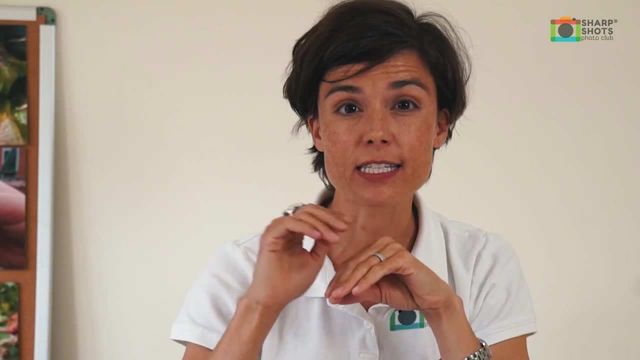 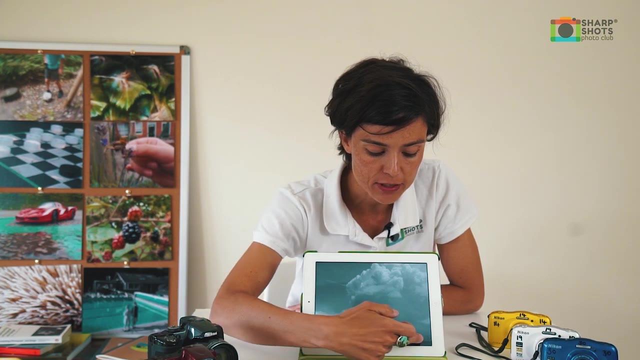 so showing that we're in your garden, but the tree or the flower is nicely in focus. So just to give you a couple of examples, a picture here: Do you see how you can see the horizon here? It's really, really low. 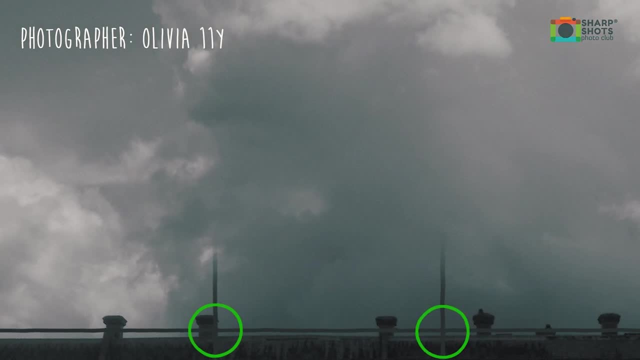 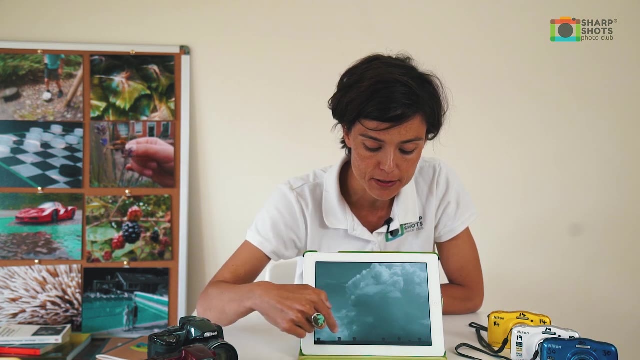 Well, instead of putting your picture right and left, you can also make sure that that horizon, where the ground meets the sky, is either the top or the bottom. So here the cloud looks really big and daunting and a very small amount of roof, Or the opposite. 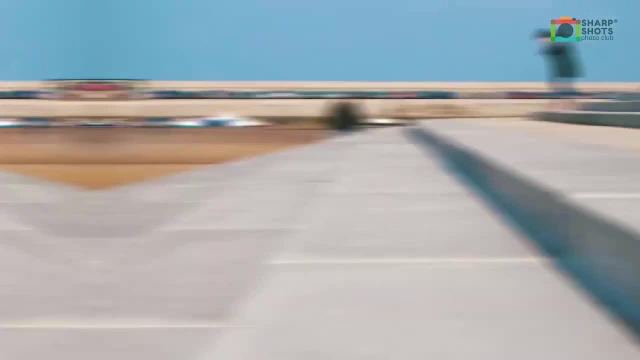 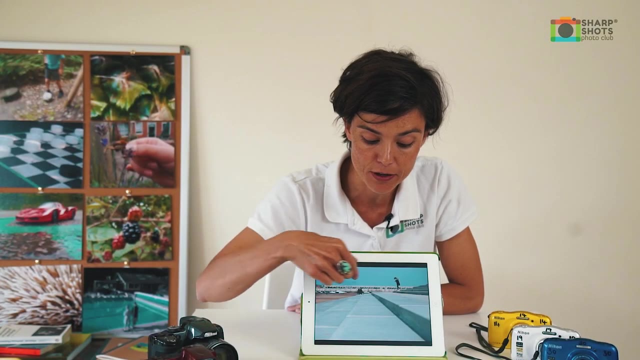 So you see, we have a lot of steps and a lot of ground and a very small amount of sky. So we're using the rule of thirds in a different way. instead of right and left, We're using it up and down. So a very third, small amount here and a large amount here. 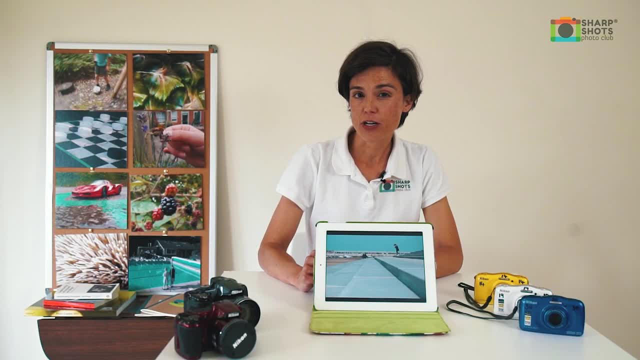 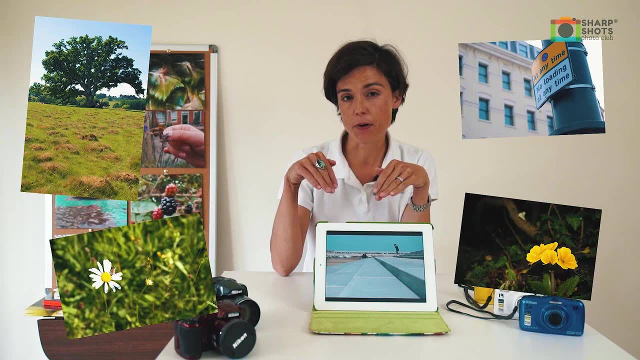 So just remember: the main thing is, when you're taking photographs using the rule of thirds, don't put your subject in the center. Try putting them up on the right or the left, or the top or the bottom, and that will really make your photographs pop. 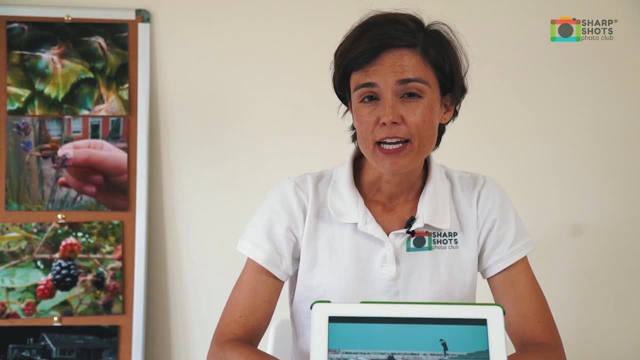 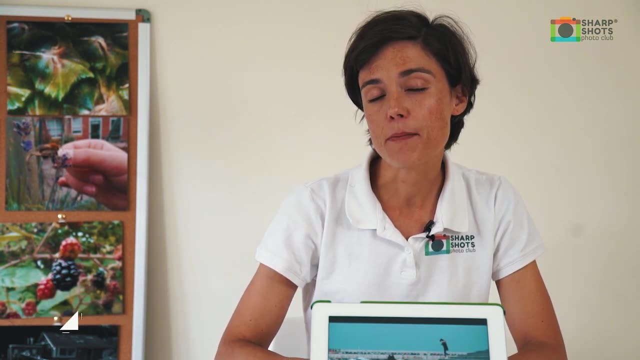 The composition will look great. Thanks for tuning in. It would be great if you could like and subscribe to our Sharp Shots Photo Club YouTube channel, And it would be really great if you could also leave us a couple of comments about what you think about our rule of thirds top tips. 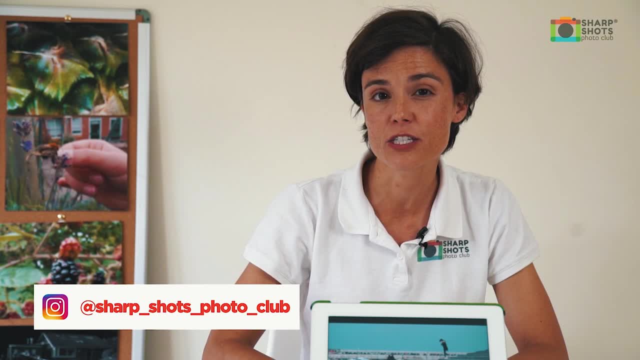 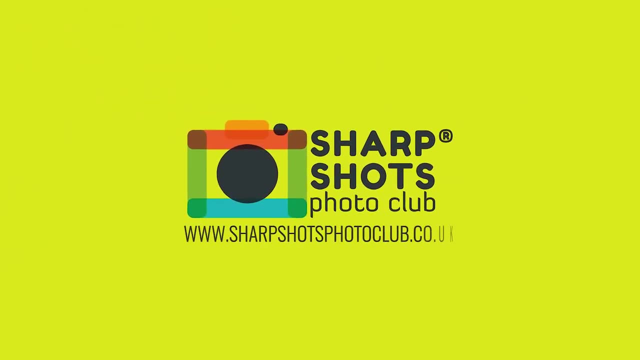 And we'd love to see the photographs that you take using the rule of thirds. So if you could tag us on Instagram, that would be wonderful. Thanks for watching and hope to see you again soon. We'll see you next time.